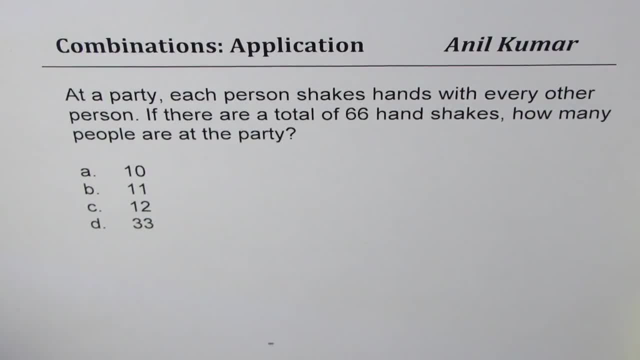 I'm Anil Kumar, sharing with you a test question on combinations At a party, each person shakes hand with every other person. If there are a total of 66 handshakes, how many people are at the party? Four choices are 10,, 11,, 12, 33.. You can always pause the video answer. 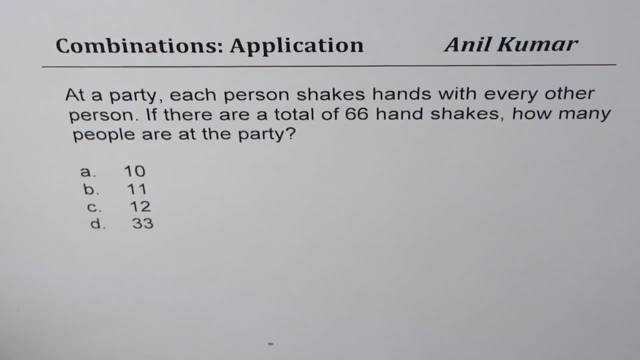 the question and then look into my suggestions. Let's go through this question once again. At a party, each person shakes hand with every other person. If there are a total of 66 handshakes, how many people are at the party? So let us say number of persons at the party are N. 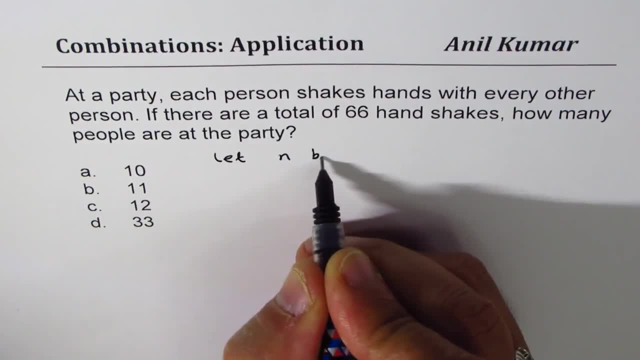 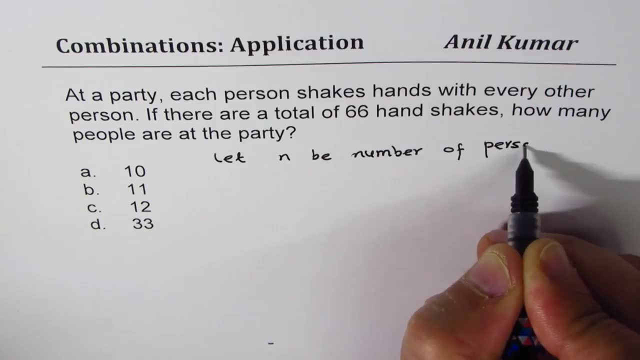 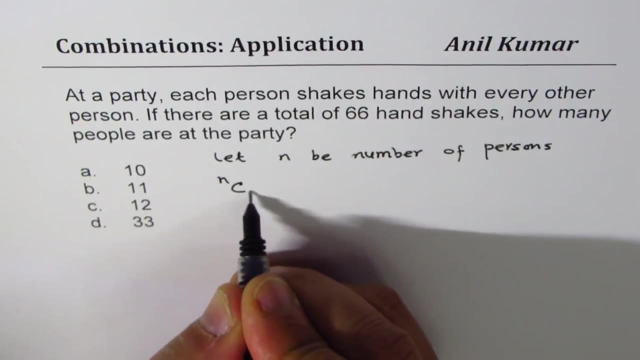 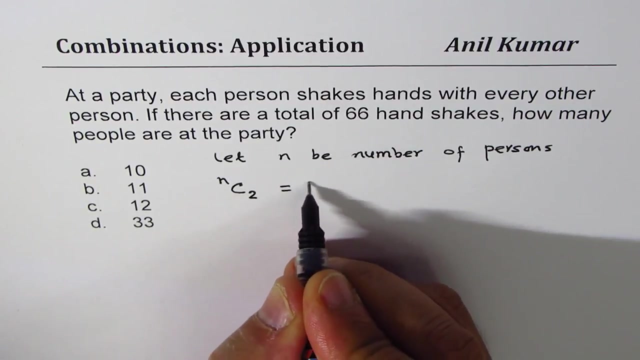 So let N be number of persons. Now, when we are talking about handshakes, it is always between two persons, So it is a combination of N persons taken two together, right? So it is NC2, whose value is 66. So 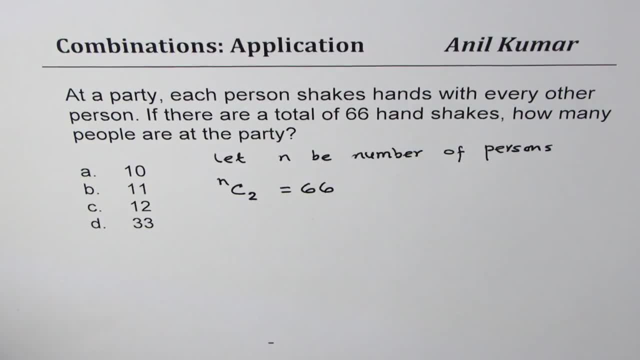 that is how you could make an equation and then solve for it. Now, NC2 is N factorial over N. N factorial is 2 factorial times N minus 2 factorial, and that is 66. So we could write this as N factorial. We could write this as N times N minus 1 times N minus 2 factorial. 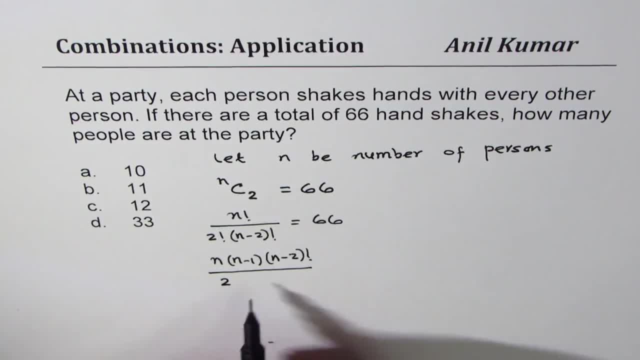 over 2 factorial is 2 times N minus 2 factorial. So n minus 2 factorial cancels out all this is equal to 66.. So we get a quadratic equation which is n times n minus 1 over 2 equals to 66, right. 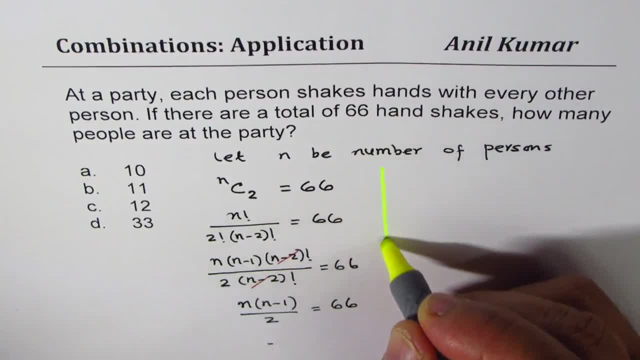 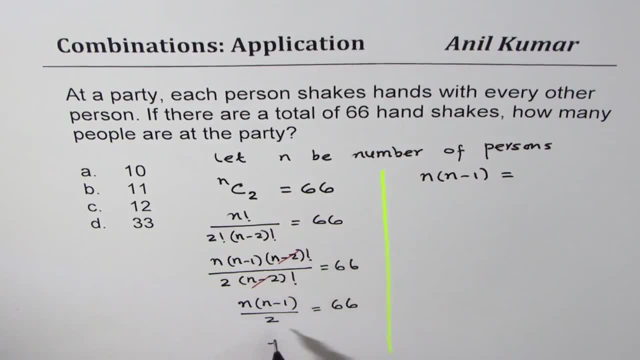 So let me take this equation to the right size and then solve for it. So the equation is n times n minus 1 equals to: we'll cross multiply so we get 66 times 2.. Let's open the bracket n square minus n. 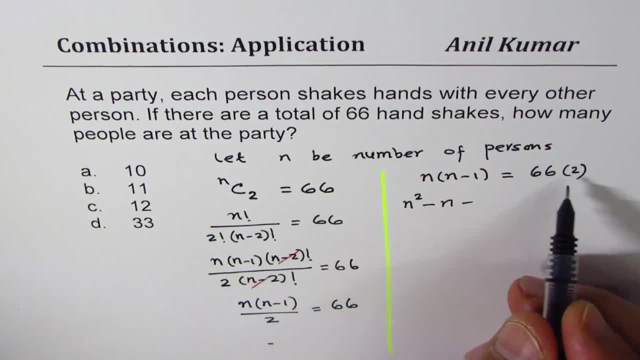 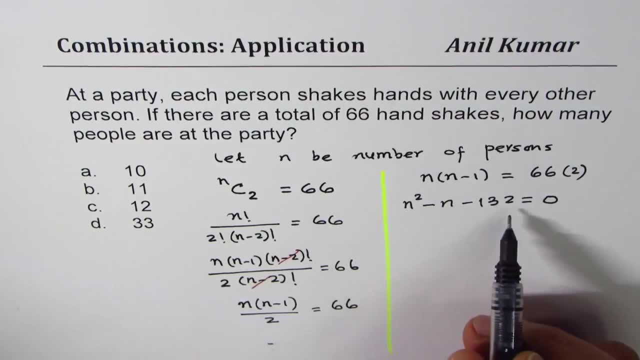 Bring this term to the left side: 66 times 2 is 132, equals to 0.. You could use quadratic formula or factor this: 12 times 11 is 132. So we could factor this as n minus 12,, since this is minus n times n plus 11.. 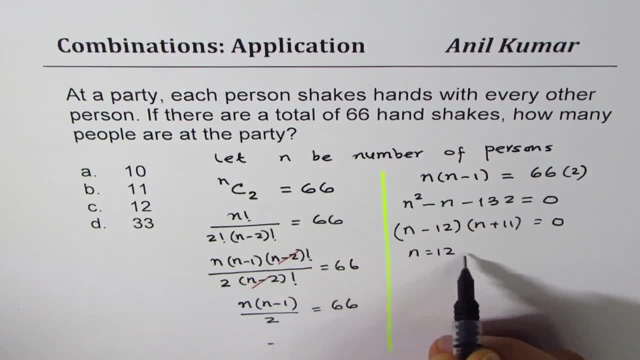 Equals to 0. That gives you n as equals to 12, or n equals to minus 11.. Now that is not valid. So the only valid answer is n equals to 2, 12.. So the option C is the correct option, and that is how it could be solved. 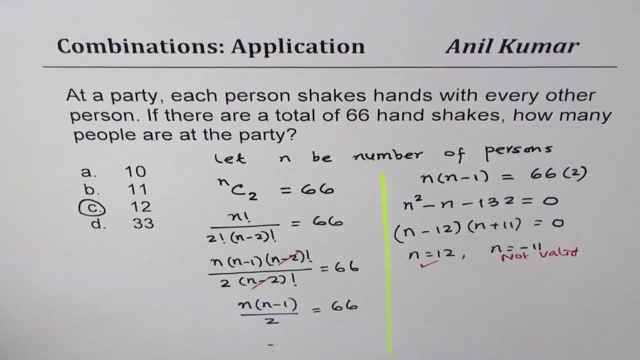 I hope that helps. Thanks and all the best. 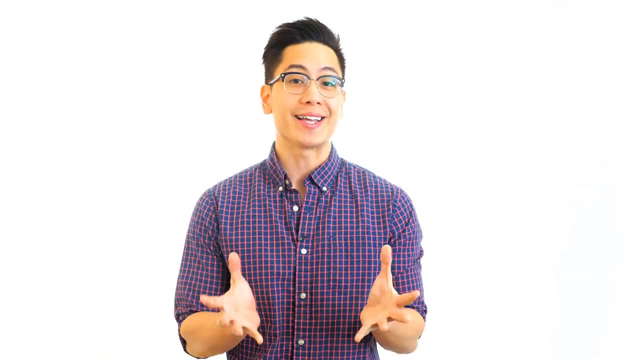 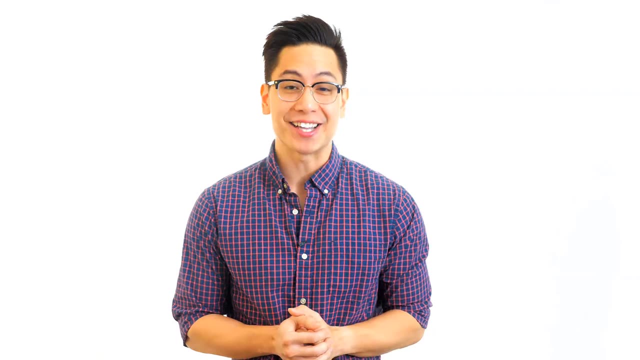 Hi and welcome. We at 365 Data Science specialize in data science trainings. We post videos weekly so you can master indispensable skills for free. Alright, let's get started. Conditional probability is the likelihood of an event occurring, assuming a different one has. 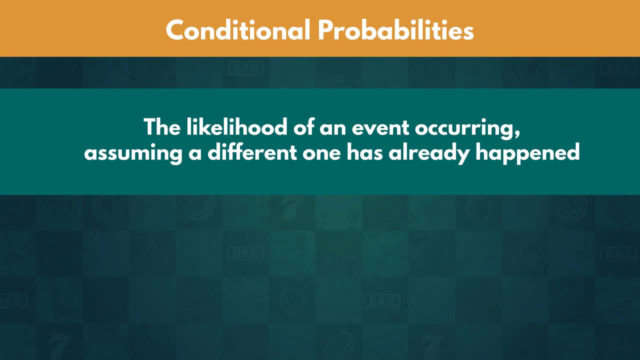 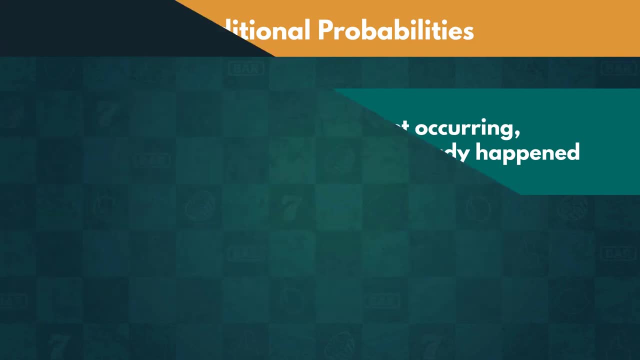 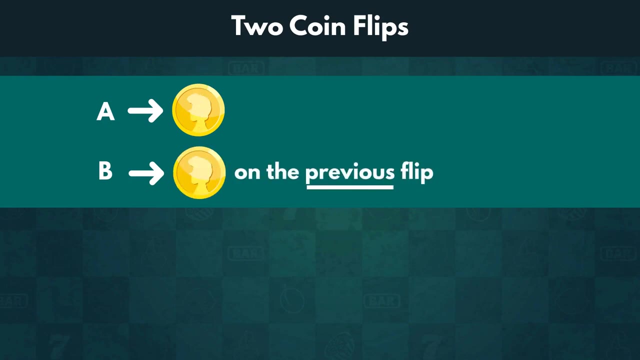 already happened. In this lecture we are going to show you how to compute and interpret such probability. Let's go back to the coin flip example from the last lecture. A represents getting heads and B represents getting heads on the previous flip. The probability of getting heads now, after getting heads last time, is still 0.5. 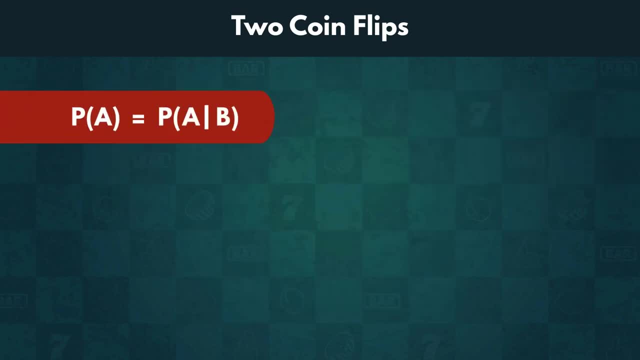 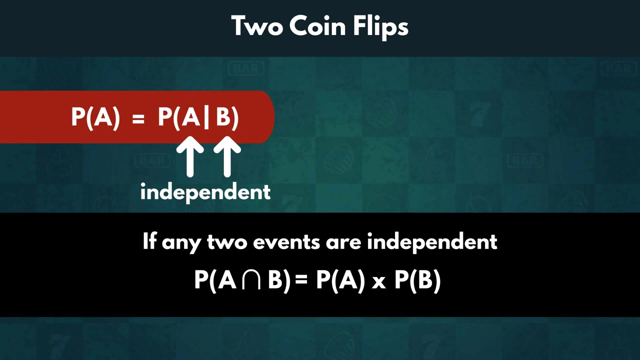 Therefore, P of A equals P of A given B. This is equivalent to saying the two events are independent. Earlier in the course we also mentioned that if any two events are independent, the probability of their intersection is the product of the individual probabilities. Now let us examine the queen of spades example.